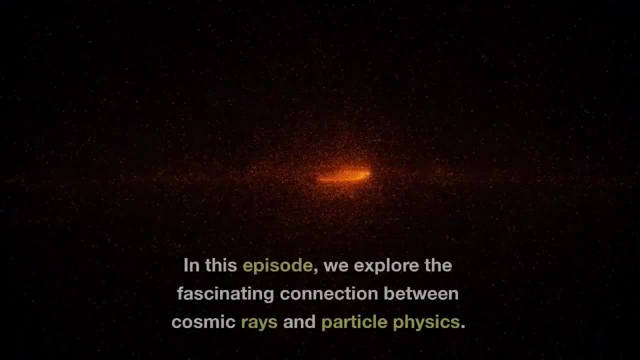 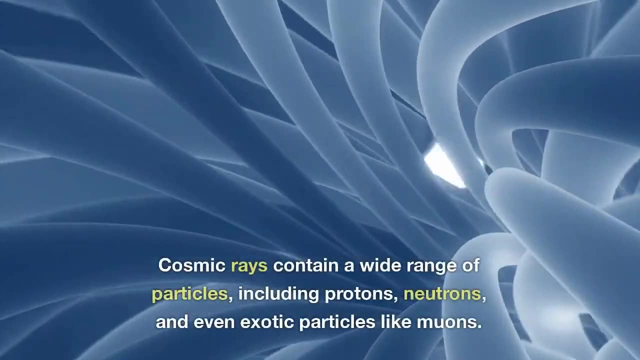 universe感覺, nutria and galaxy and friendships. cosmic rays and particle physics. We explore the fascinating connection between cosmic rays and particle physics. In this episode, we explore the fascinating connection between cosmic rays and particle physicsval الله. Cosmic rays contain a wide range of particles, including protons, neutrons and even exotic particles like muons. 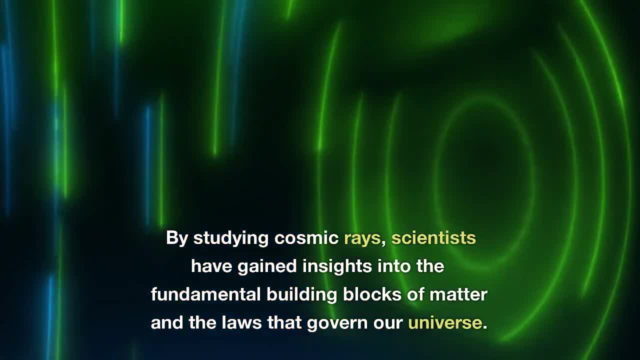 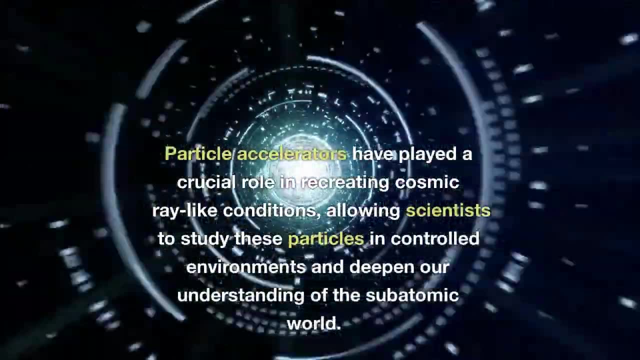 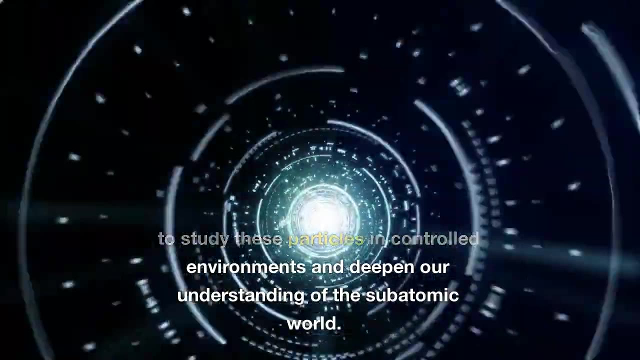 By studying cosmic rays, scientists have gained insights into the fundamental building blocks of matter and the laws that govern our universe. Particle accelerators have played a crucial role in recreating cosmic ray-like conditions, allowing scientists to study these particles in controlled environments and deepen our understanding of the subatomic world. 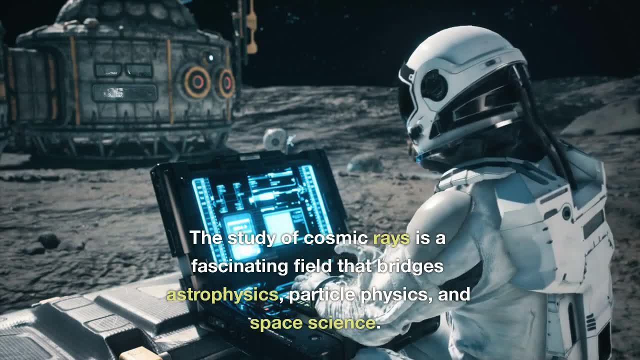 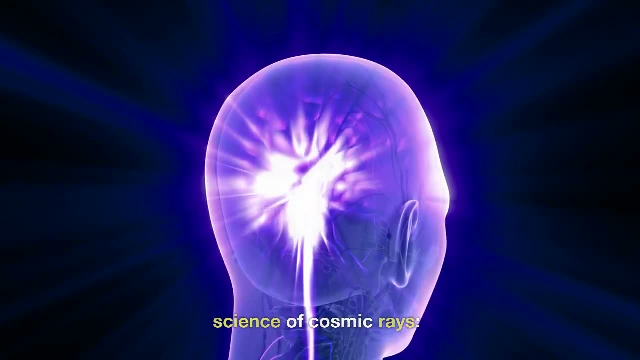 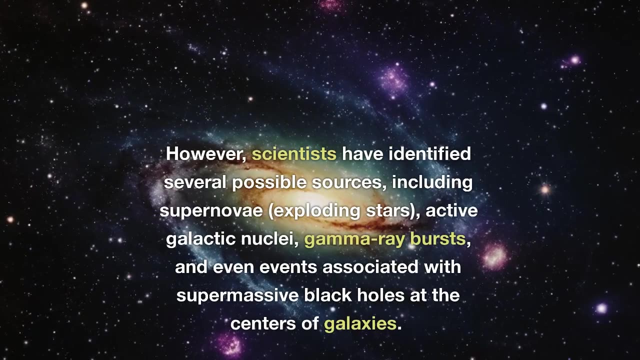 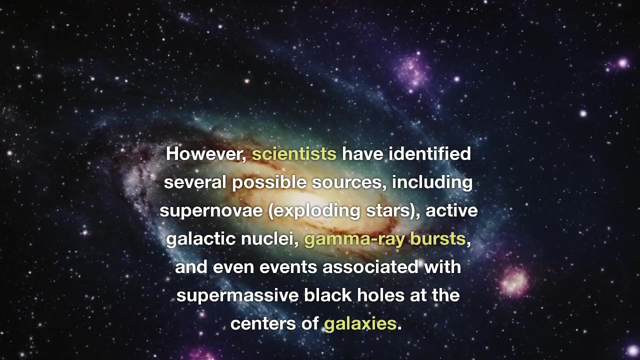 The study of cosmic rays is a fascinating field that bridges astrophysics, particle physics and space science. Here are some key details about the science of cosmic rays Origin. The exact sources of cosmic rays are still under investigation. However, scientists have identified several possible sources, including supernovae, exploding stars, active galactic nuclei, gamma-ray bursts. 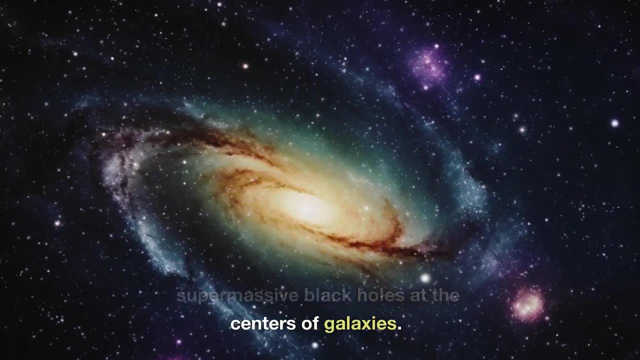 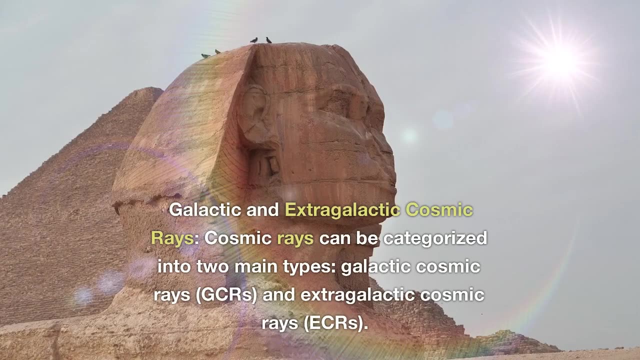 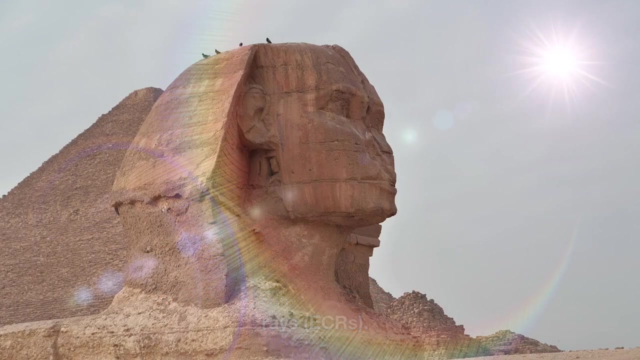 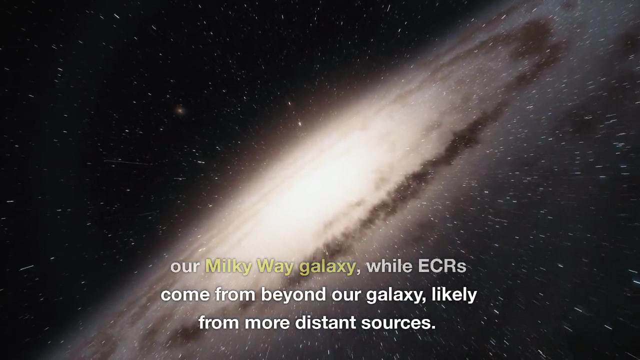 and even events associated with supermassive black holes at the center. The galaxy's galactic and extragalactic cosmic rays can be categorized into two main types. Galactic cosmic rays and extragalactic cosmic rays are believed to originate within our Milky Way galaxy, while ECRs come from beyond our galaxy, likely from more distant sources. 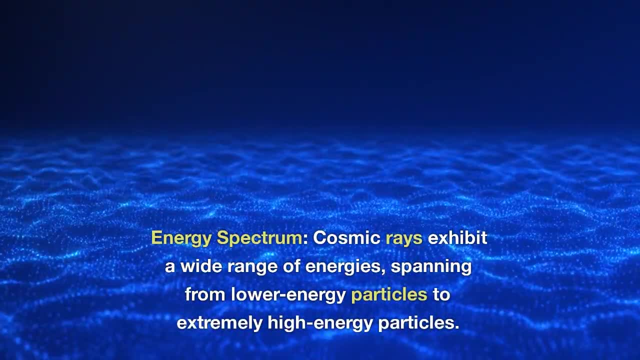 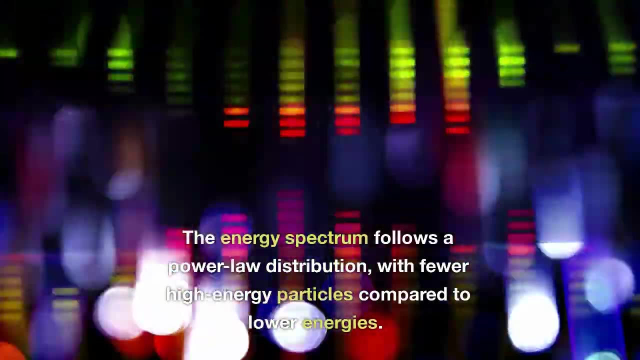 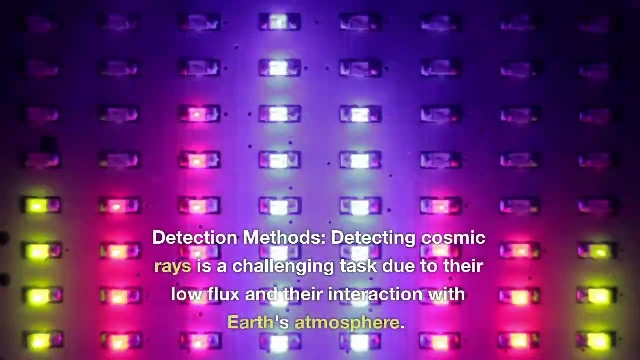 Energy spectrum. Cosmic rays exhibit a wide range of energies, spanning from lower energy particles to lower energy particles. The energy spectrum follows a power law distribution, with fewer high-energy particles compared to lower energies. Detection methods: Detecting cosmic rays is a challenging task due to their low flux and their interaction with Earth's atmosphere. 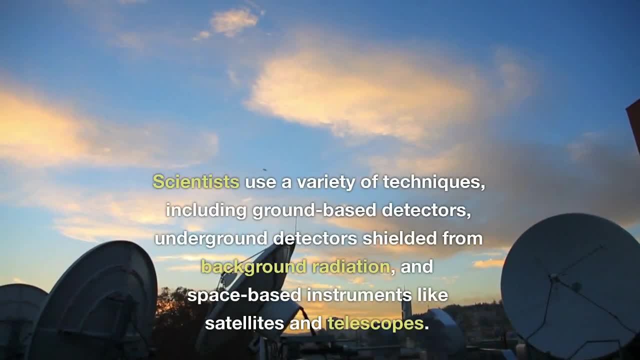 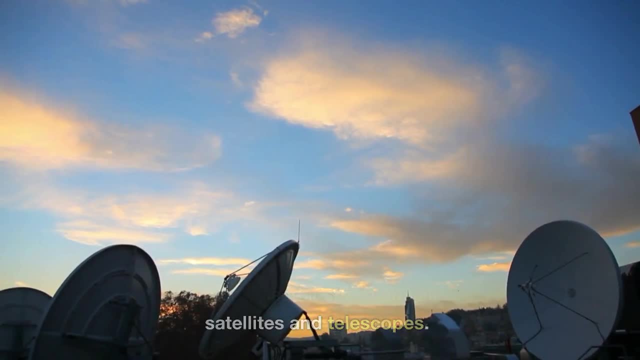 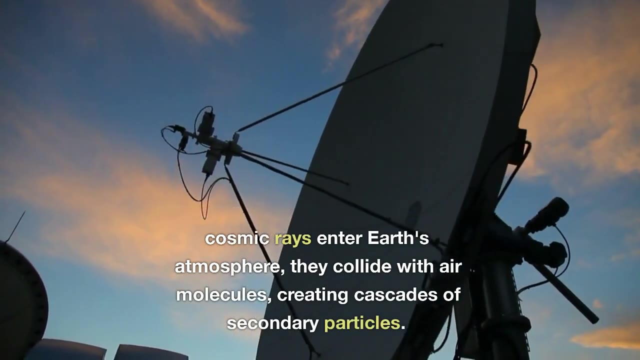 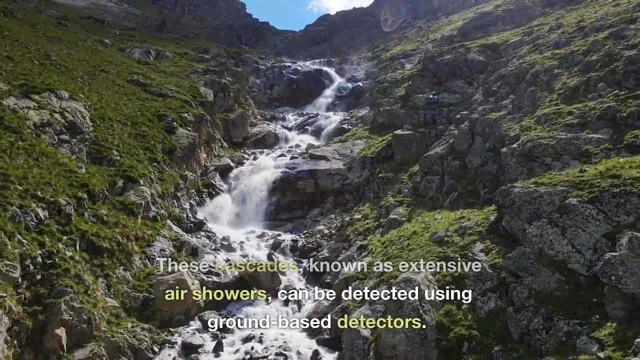 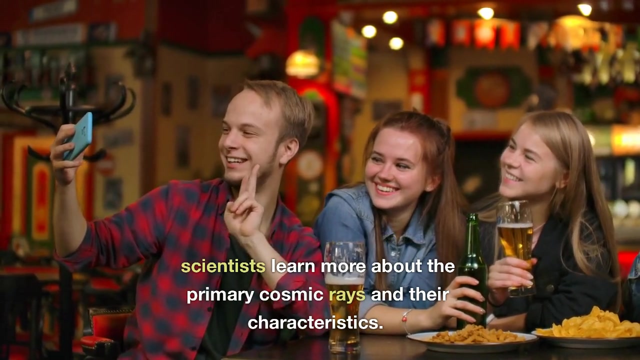 Scientists use a variety of techniques, including ground-based detectors, underground detectors shielded from background radiation, and space-based instruments like satellites and telescopes. Impact on Earth's Atmosphere. When cosmic rays enter Earth's atmosphere, they collide with air molecules, creating cascades of secondary particles. These cascades, known as extensive air showers, can be detected using ground-based detectors. Studying these showers helps scientists learn more about the primary cosmic rays and their characteristics. 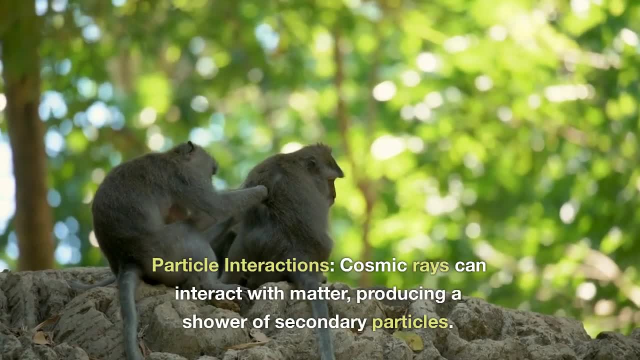 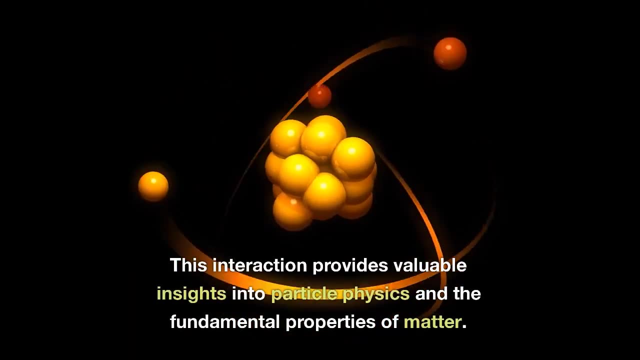 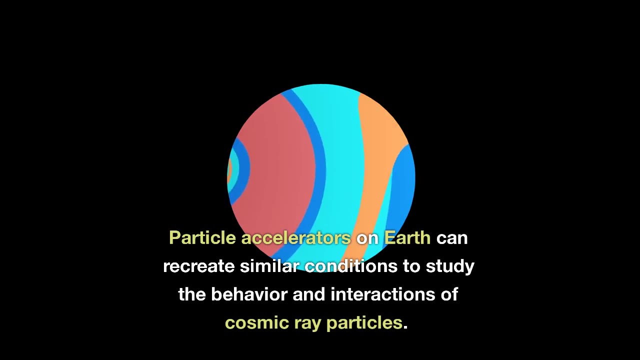 6. Particle Interactions. Cosmic rays can interact with matter, producing a shower of secondary particles. This interaction provides valuable insights into particle physics and the fundamental properties of matter. Particle accelerators on Earth can recreate similar conditions to study the behavior and interactions of cosmic ray particles. 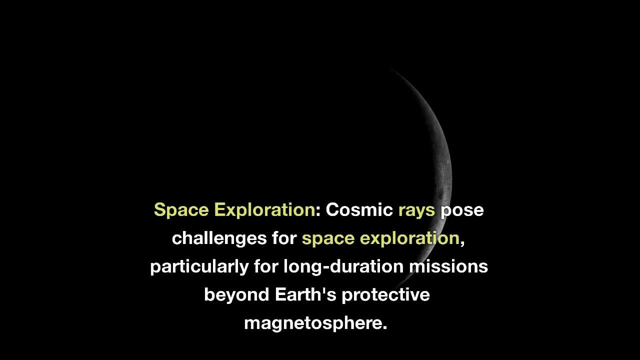 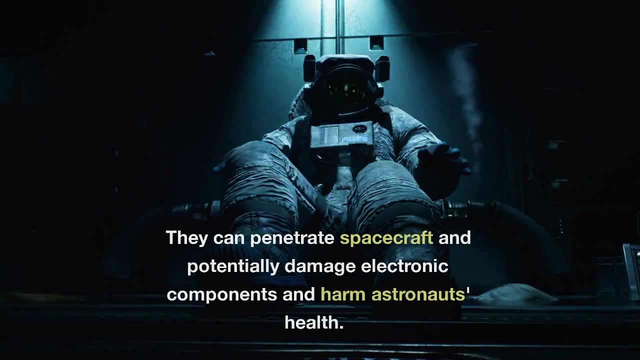 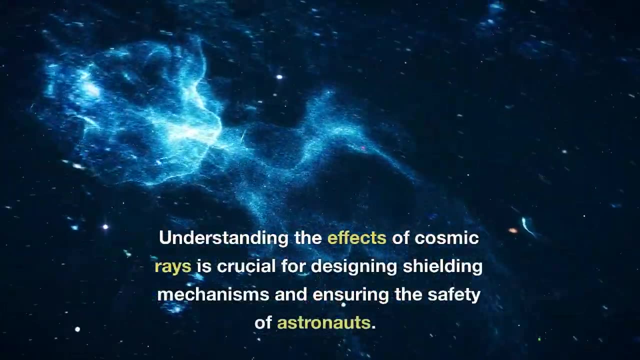 7. Space Exploration. Cosmic rays pose challenges for space exploration, particularly for long-duration missions beyond Earth's surface. They can penetrate spacecraft and potentially damage electronic components and harm astronauts' health. Understanding the effects of cosmic rays is crucial for designing shielding mechanisms and ensuring the safety of astronauts. 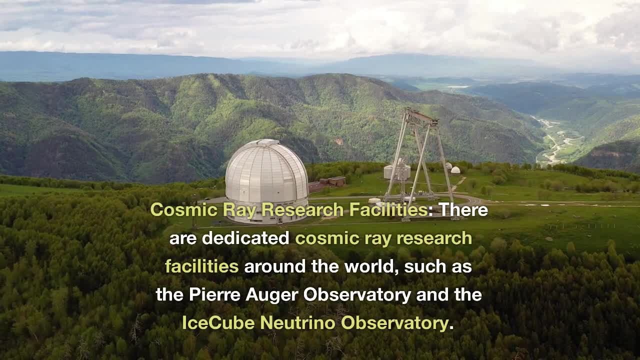 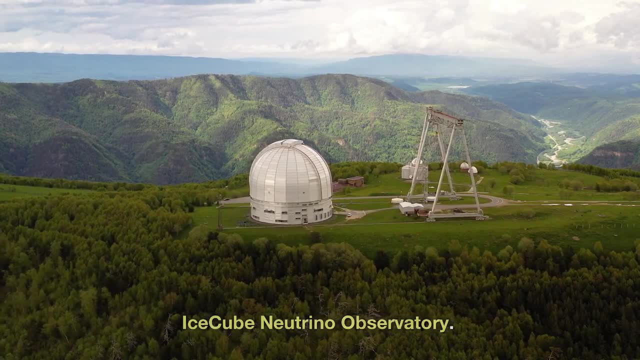 8. Cosmic Ray Research Facilities. There are dedicated cosmic ray research facilities around the world, such as the Pierre Auger Observatory and the IceCube Neutrino Observatory. These facilities aim to study cosmic rays in different energy regions. They can gather new and advanced some of the largest cosmic rays on Earth's surface and create new challenges that create potential for space exploration. 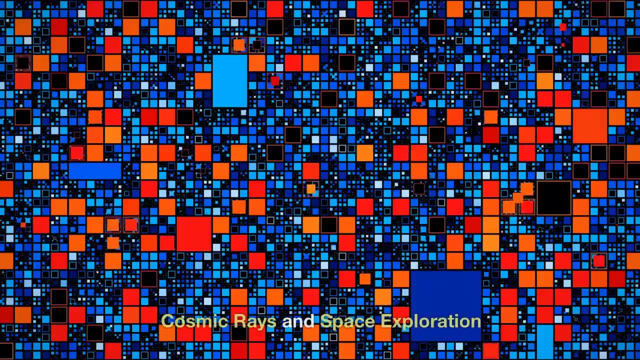 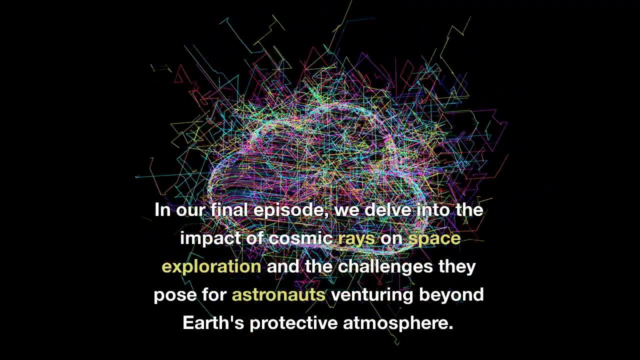 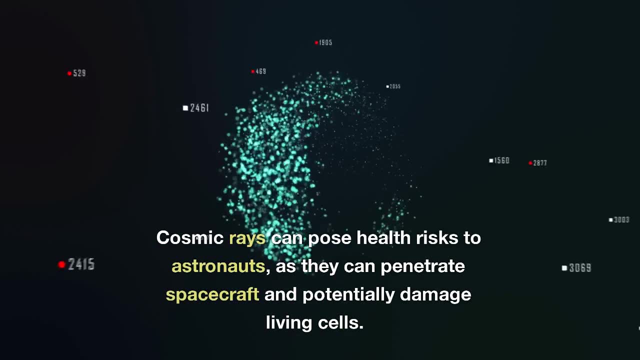 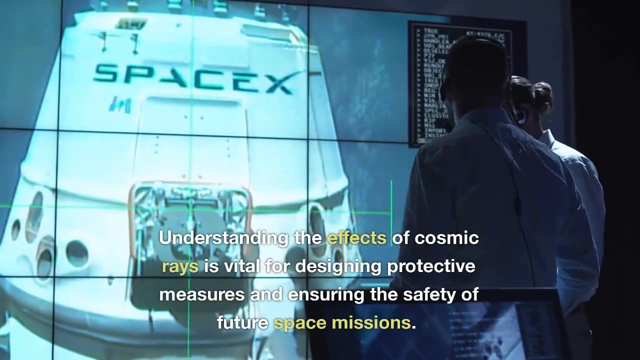 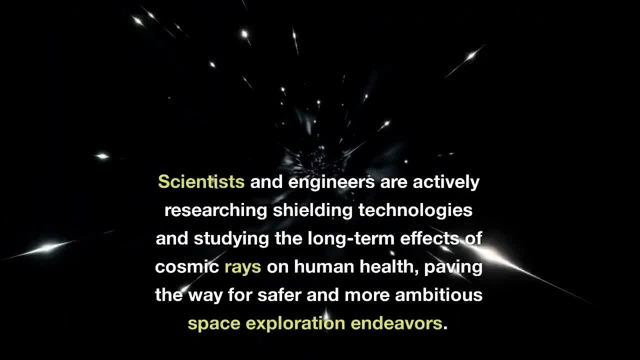 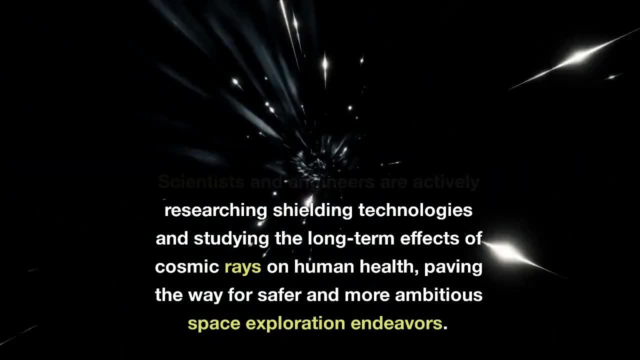 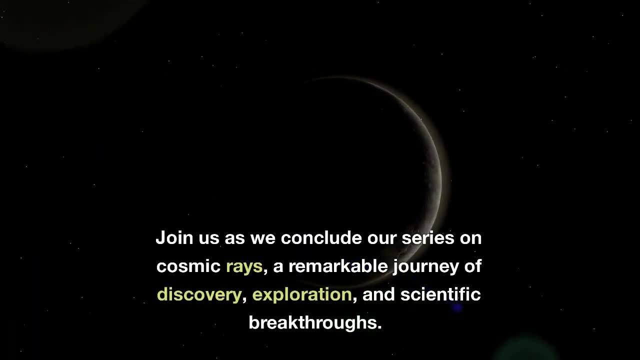 Or mu, ensuring the safety of future space missions. Scientists and engineers are actively researching shielding technologies and studying the long-term effects of cosmic rays on human health, paving the way for safer and more ambitious space exploration endeavors. Join us as we conclude our series on Cosmic Rays: a remarkable journey of discovery exploration. 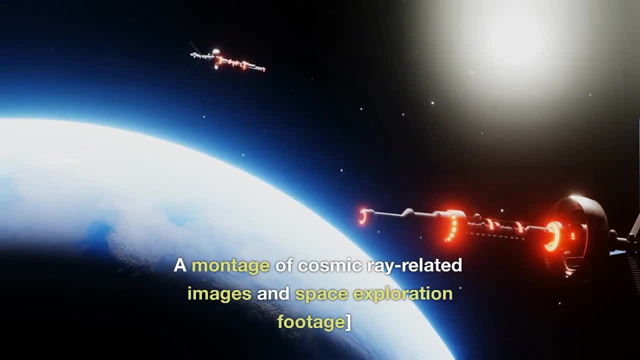 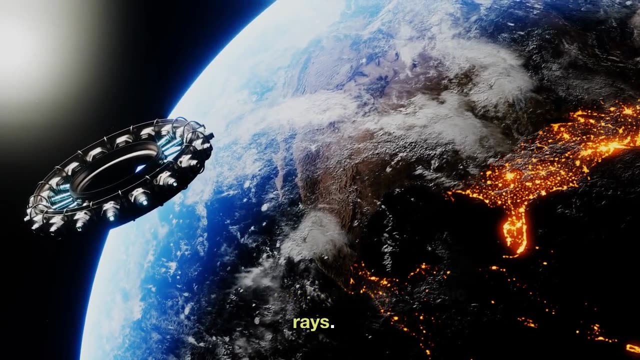 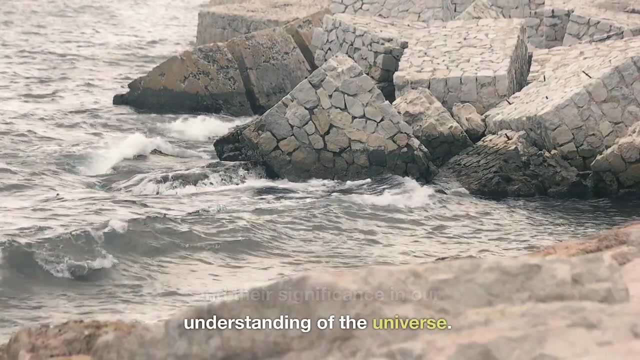 and scientific breakthroughs. A montage of cosmic ray-related images and space exploration footage. Thank you for joining us on this captivating exploration of cosmic rays. Together, we've uncovered the mysteries of these energetic particles and their significance in our understanding of the universe. 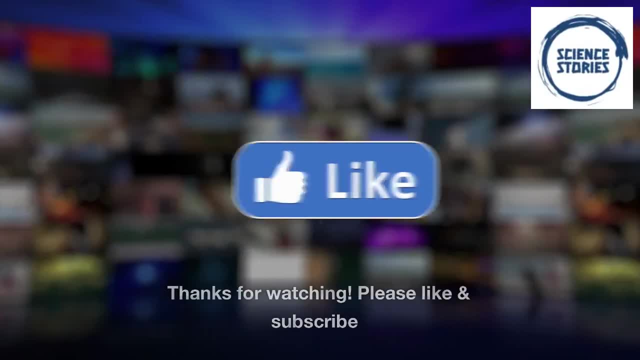 Stay curious and keep exploring the wonders of science. Thanks for watching. Please like and subscribe.